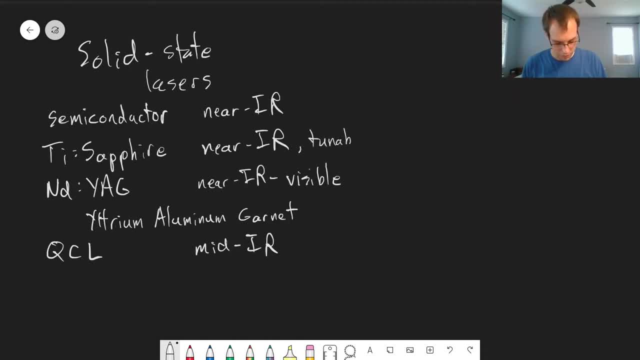 Titanium, sapphire is near IR and also tunable Liquid. we also have liquid-based lasers, And there's essentially only one, though it's a very important one- is the dye laser. And what's useful with the dye laser is this can range all the way from visible to UV with different laser. 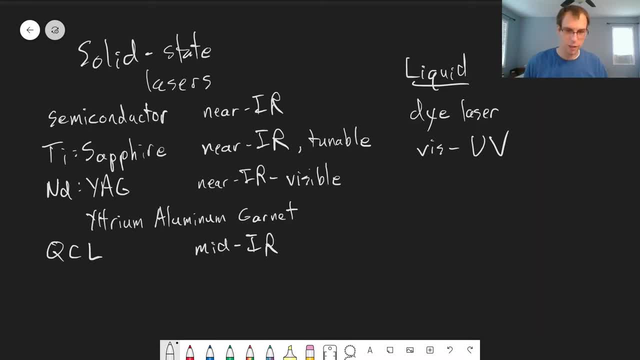 dyes that you can use, And so I used a liquid-based dye laser in my postdoc. And then we also have gas phase lasers, So basically we kind of classify them by the state of the lasing medium, And so one of the most common ones, gas phase, is the helium neon laser or HENI. 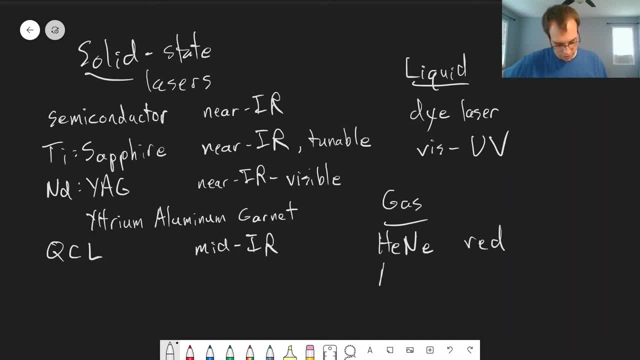 This emits specifically red light. There's an argon ion laser, nitrogen laser, CO2 lasers and another one, eczema, an excited dimer laser. So CO2 works in the infrared, N2 is UV, argon is visible and eczema lasers work in the UV. 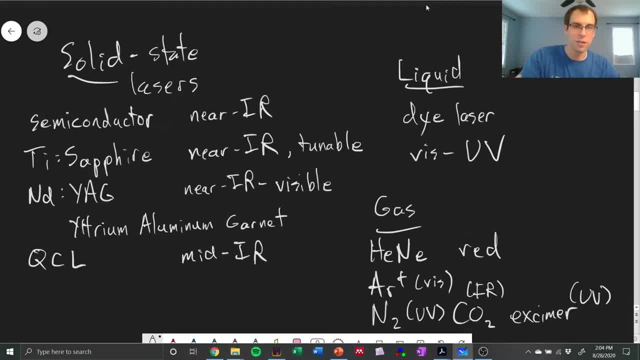 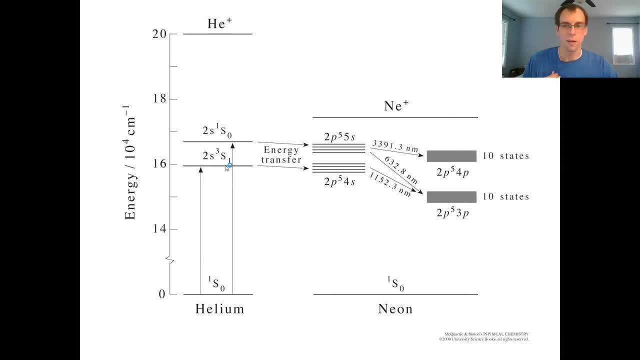 So just to, I have a couple pictures I want to show in this PowerPoint here. So there we go. So we have here. this is the energy level diagram for a helium neon laser. So it's a combination of these two. So you actually excite the helium, but the helium transfers its energy to the neon. 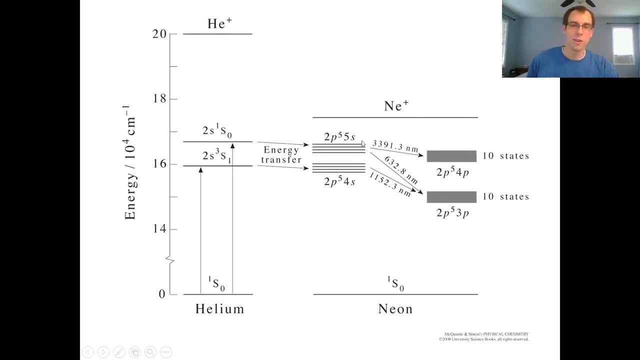 and that generates our population inversion, And so there's actually multiple different lasing transitions that can be used. The most common one is this one here, at 632.8 nanometers, And so this: you generate an electrical discharge inside of a mixture of helium and neon gas. 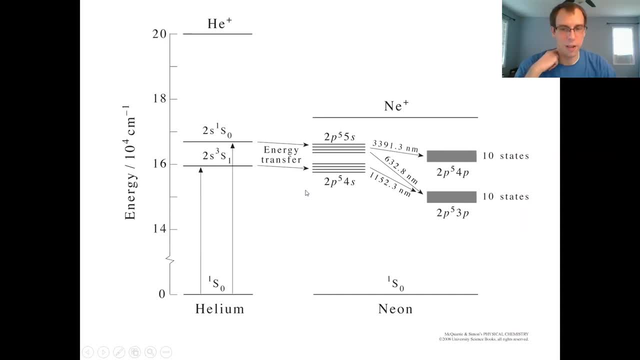 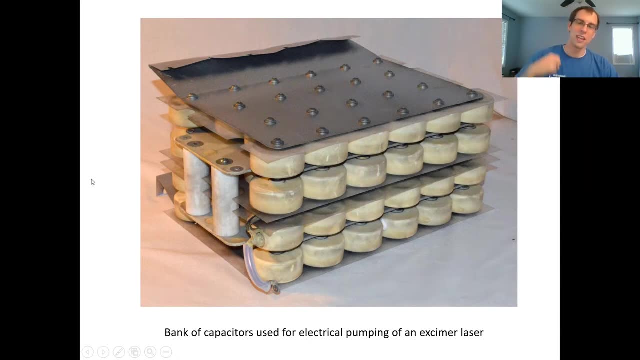 and that generates the, the lasing medium. and then you have your mirrors and output coupler. so eczema lasers are interesting. they also use electrical pumping and they use these giant banks of capacitors, so I worked with these. they're a little bit scary because they can. 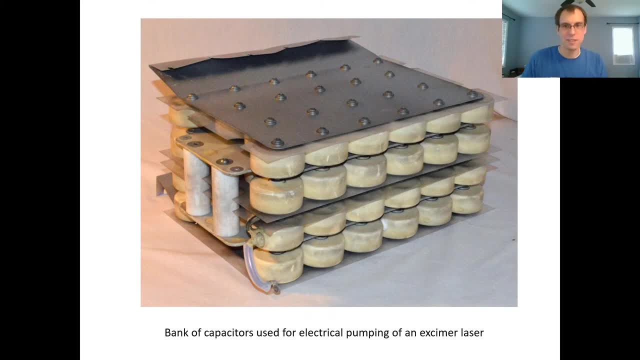 store a lot of electricity and you need a lot of electricity all at once to generate the the laser and for an eczema laser, and so these are about hockey puck sized each of these and they can explode. so I've spent a lot of time during my two years in Atlanta changing these out as